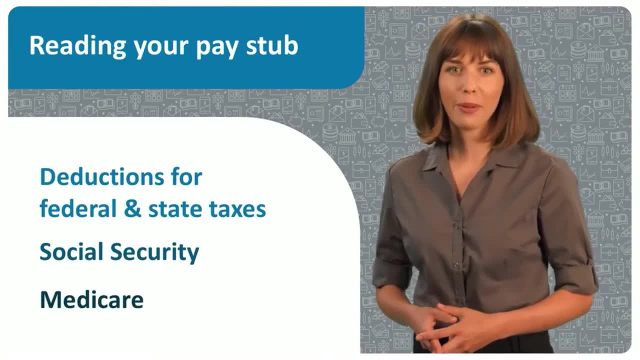 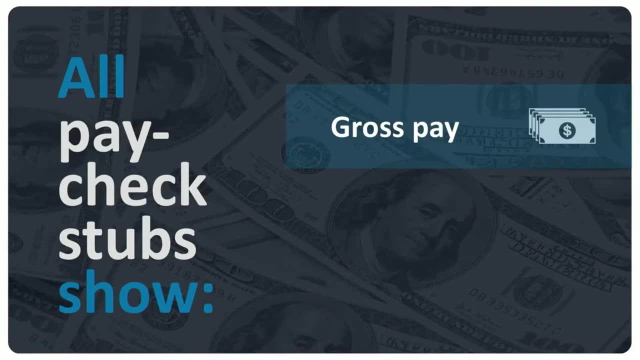 we're going to focus on the taxes that you'll commonly see on your pay stub. All paycheck stubs show your gross pay, the total amount you earned before any taxes were withheld for the pay period. They also show your net pay, the amount of your check after all withholdings. Let's break. 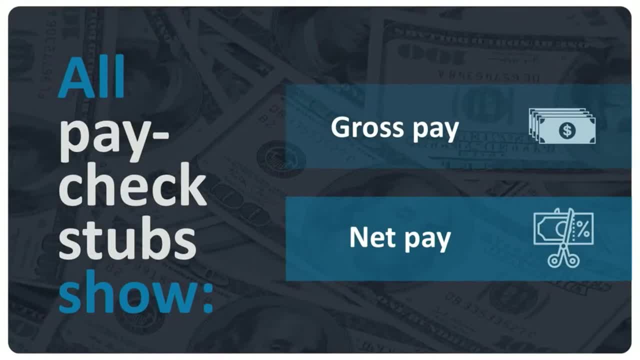 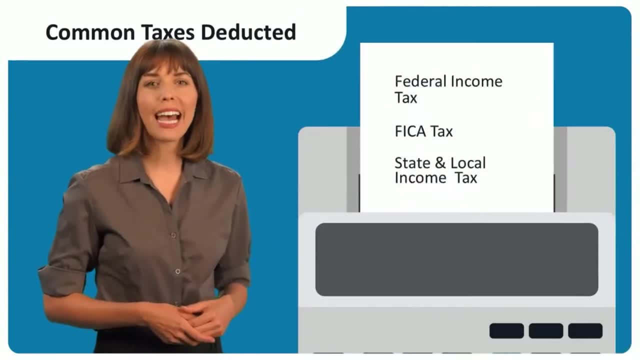 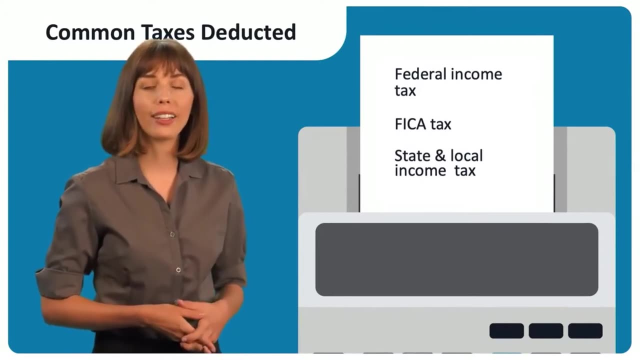 it down further in an attempt to help you better manage your money. Usually, government agencies like the IRS and state tax departments tax your pay. Common taxes deducted include federal income tax, the employee portion of FICA tax and sometimes state and local income taxes. On the. 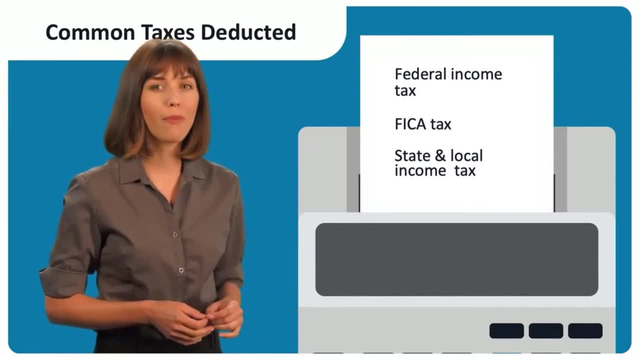 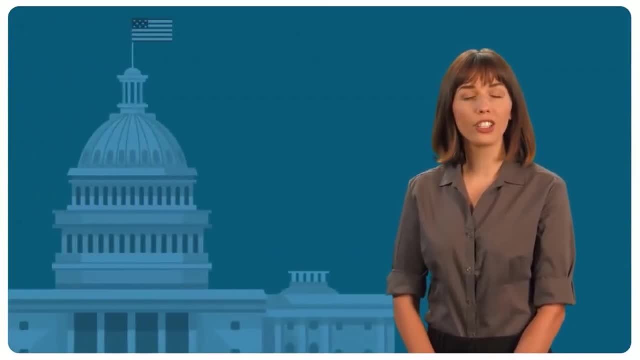 pay stub. there will be a separate line for each tax and it will show the amount deducted for the current pay period and year to date. The federal government gets a piece of your income from each and every paycheck. This piece of income is your withholding tax, the partial payment of your 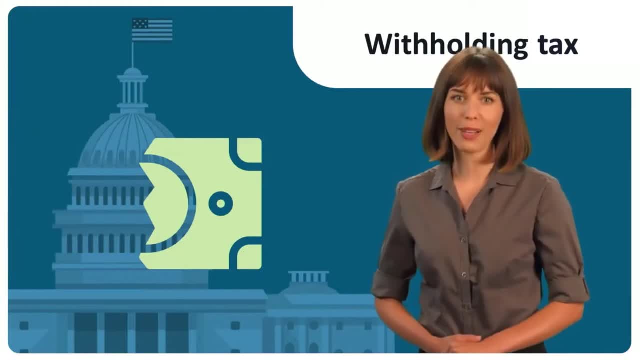 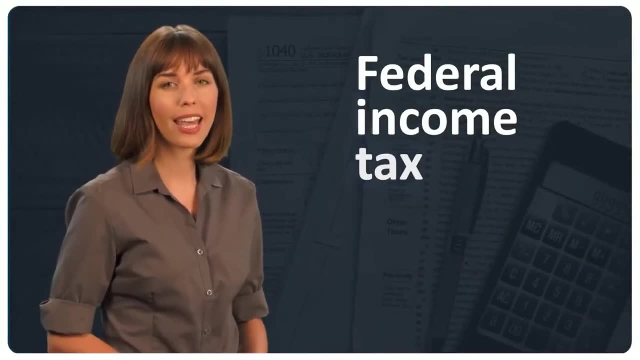 annual income taxes that get sent directly to the federal government. Federal income tax might be abbreviated as Fed tax, FT or FWT. This amount is what you've already paid the federal government, So if you're a federal government, you're going to have to pay a separate line for each tax. 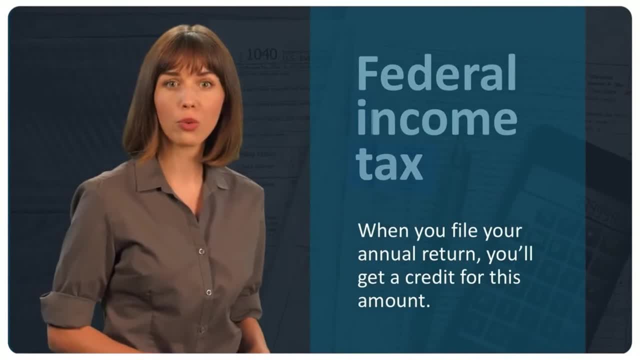 When you file your annual return, you'll get a credit for this amount to apply to any tax you might owe the federal government. The amount of money withheld for federal taxes depends on the amount of money that you earn and the information that you gave your employer when you filled out a. 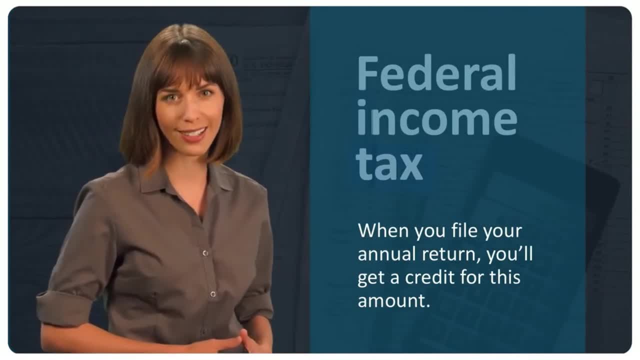 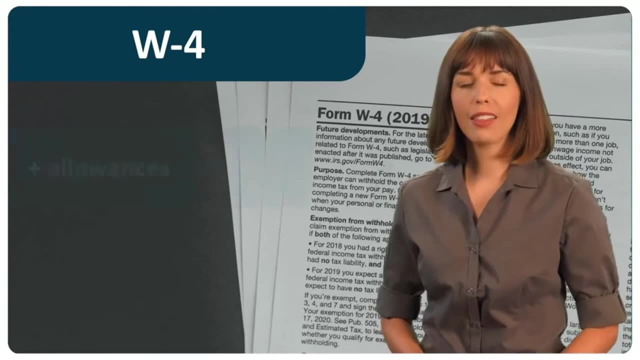 W-4 form or Employees Withholding Allowance Certificate. On a W-4, you can make allowances for yourself, your spouse and your dependents, such as your children. The more allowances you take, the less money gets withheld for federal taxes and more money gets withheld for federal taxes. 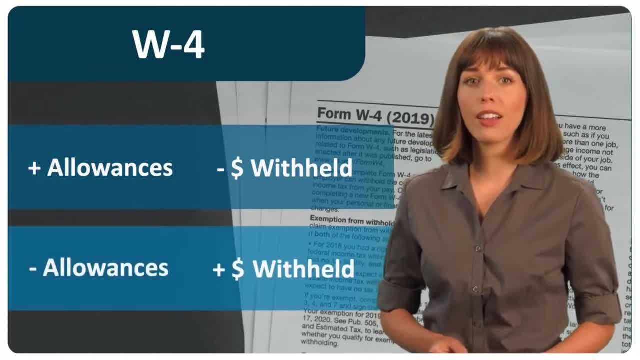 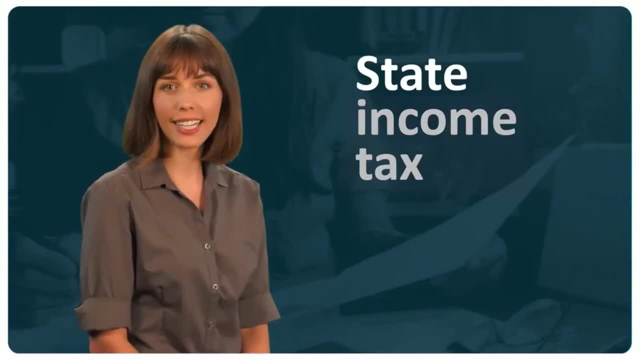 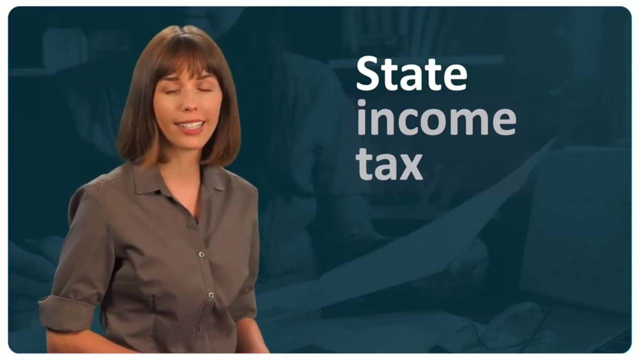 State income tax might be abbreviated as ST tax, ST or SWT. Your paycheck might also show the abbreviation of the state for which the tax is being withheld. Depending on where you live, you might not have state withholding or could have multiple withholdings for more than one. 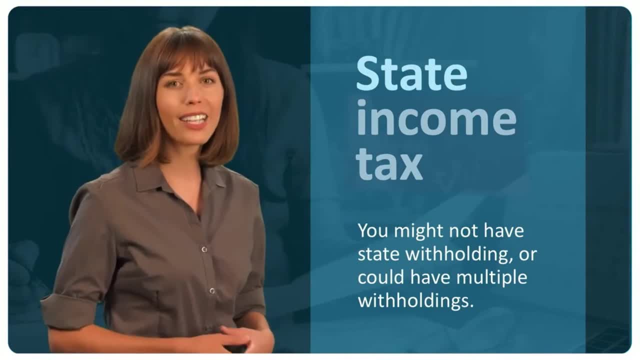 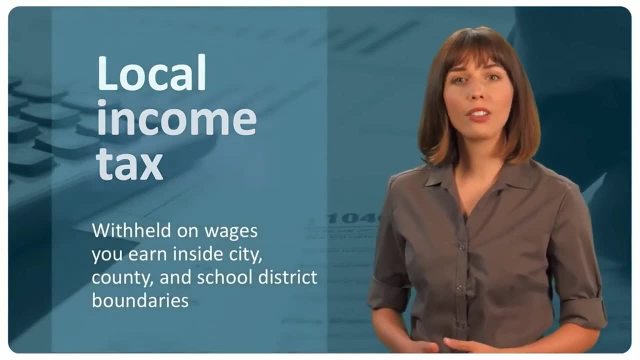 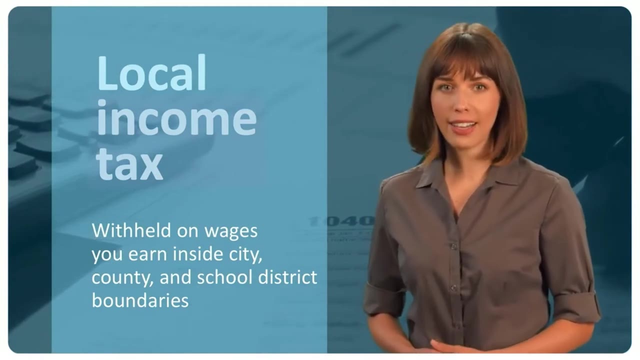 state—the state you live in and the state you work in. As with federal taxes, money for state taxes is withheld from every paycheck. Local income tax might be withheld on wages you earn inside city, county and school district boundaries If you live or work in an area that levies a tax. 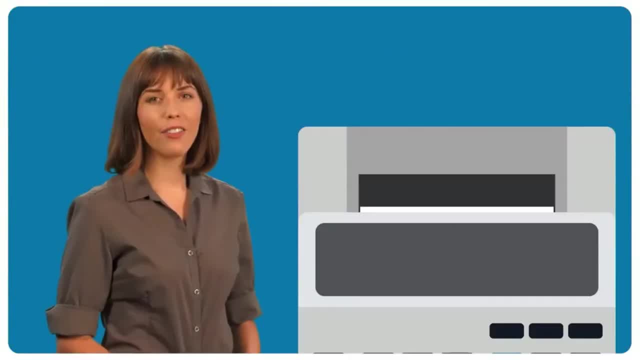 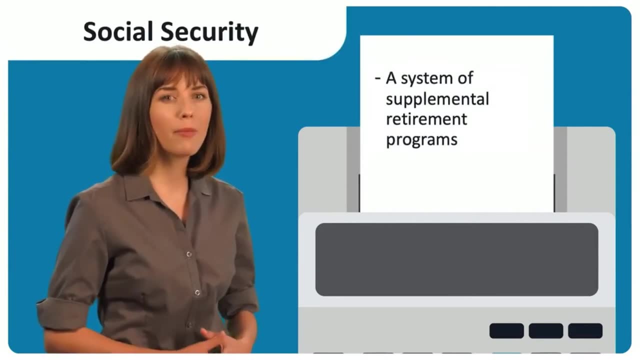 your wages will be taxed by that jurisdiction. The federal government requires every working American to contribute a portion of their paycheck to Social Security, a system of supplemental retirement programs established in 1935.. Every worker contributes 6.2% of their gross income directly into the Social Security Fund, and every employer chips in an additional. 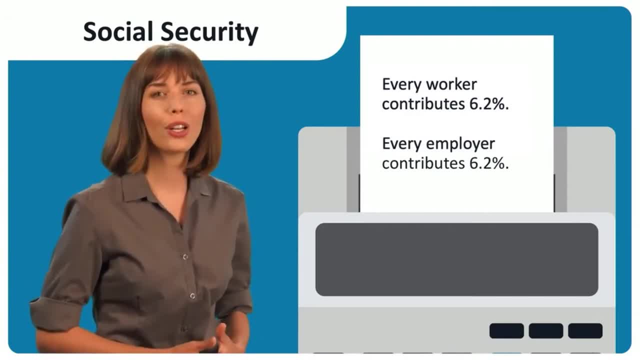 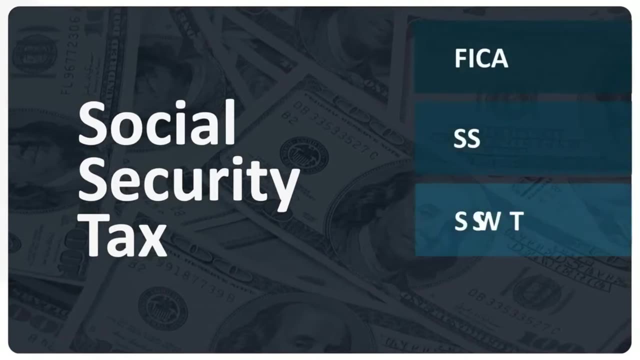 6.2% for each employee. The Social Security Fund provides benefits to current Social Security recipients. Eventually, when you're old enough, you'll be able to file for Social Security yourself. Social Security tax might be abbreviated as FICA, SS, SSWT or OASDI Usually. 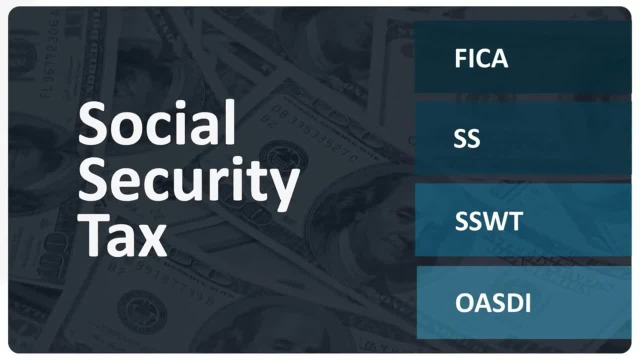 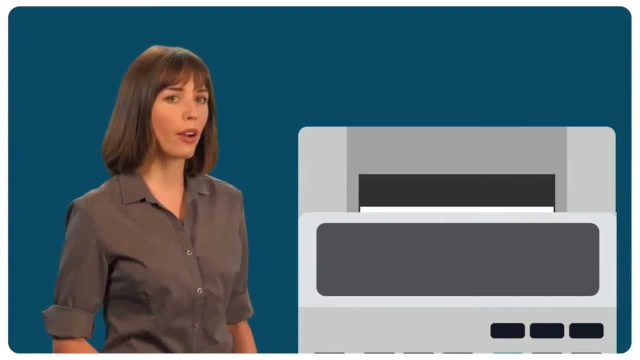 you must have these withheld. This is true even when you have nothing withheld for federal, state and local income taxes. The federal government also requires every working American to contribute to Medicare, a US government insurance plan that provides hospital, medical and surgical benefits for 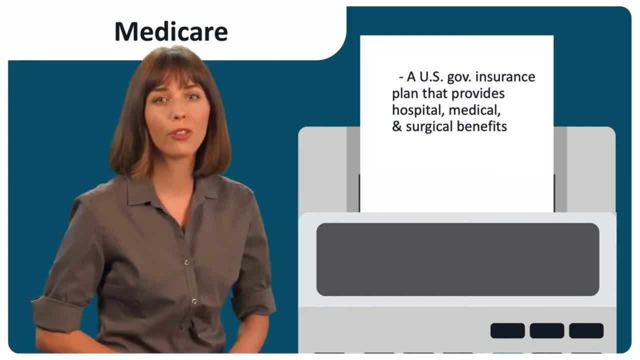 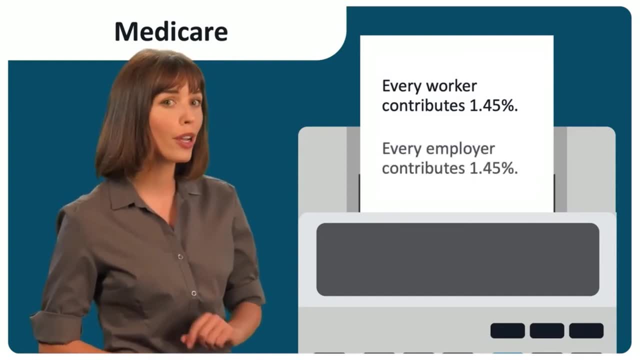 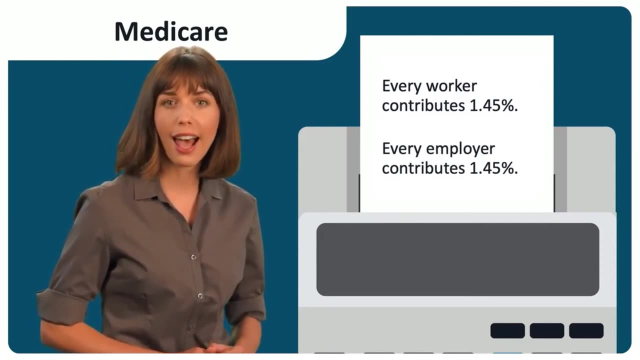 Americans ages 65 and older and for people with certain disabilities. Every worker contributes 1.45% of their gross income to Medicare and every employer pays an additional 1.45% on behalf of each employee. Medicare tax might be abbreviated as MWT or MED. 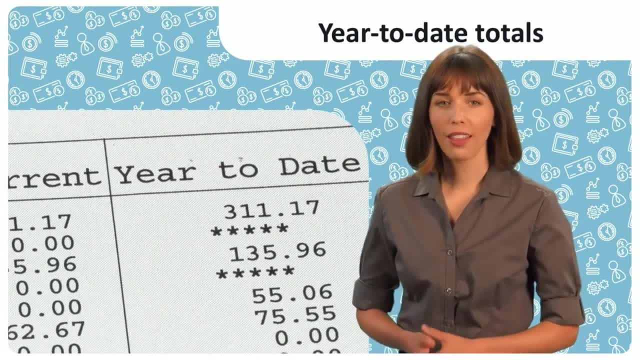 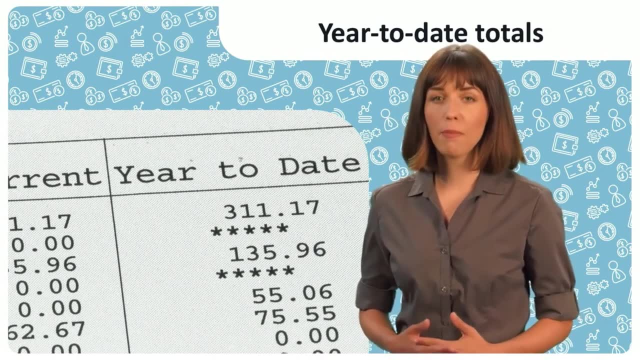 Your paycheck stub will also show year-to-date totals. This is good to know if you want to estimate if you'll have a refund or balance due at the end of the year. Save the last paycheck stub to compare with your W-2.. The amounts on the last stub and 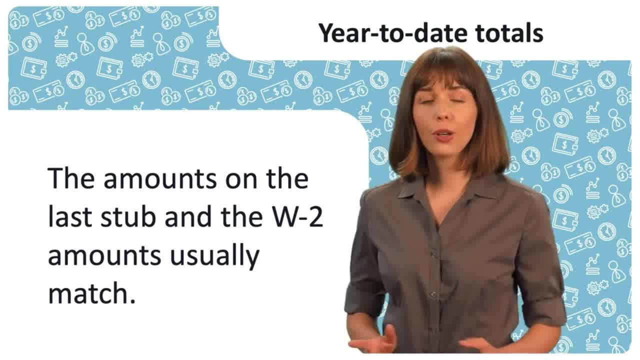 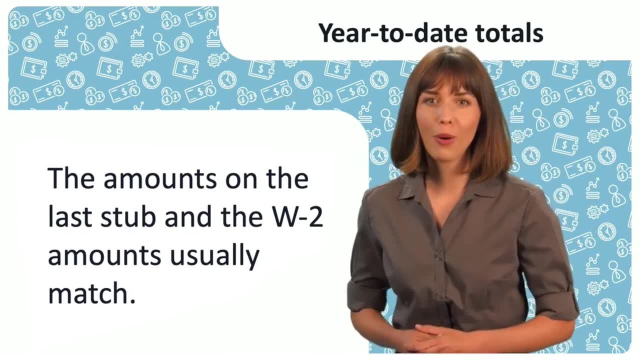 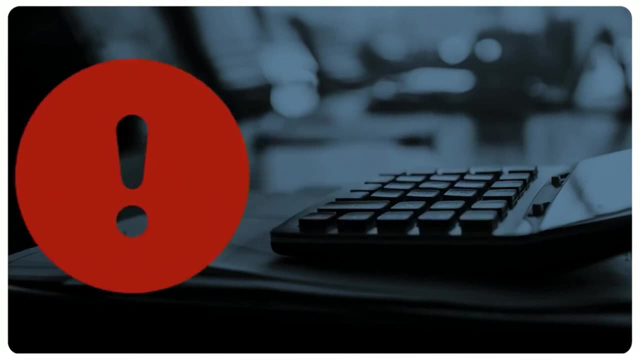 the W-2 amounts usually should match. However, your employer might have added other amounts for additional benefits offered. These could be taxable income for you. Contact your payroll department if there are any differences. It's important to be aware of the tax information on your pay stub. Any errors are your responsibility to find and report to your 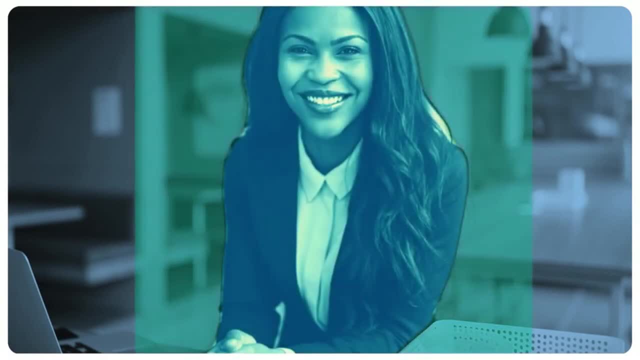 company's Human Resources department. If you have any questions about any of the information listed on your pay stub, be sure to contact Human Resources.